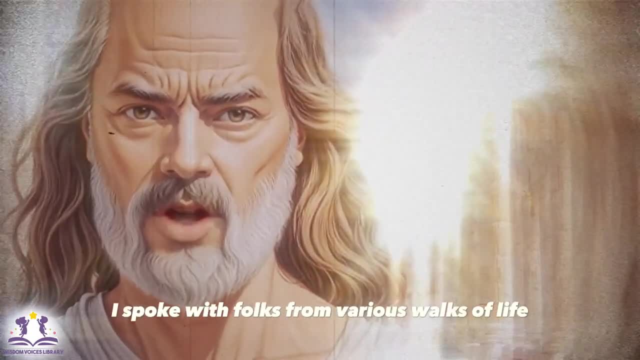 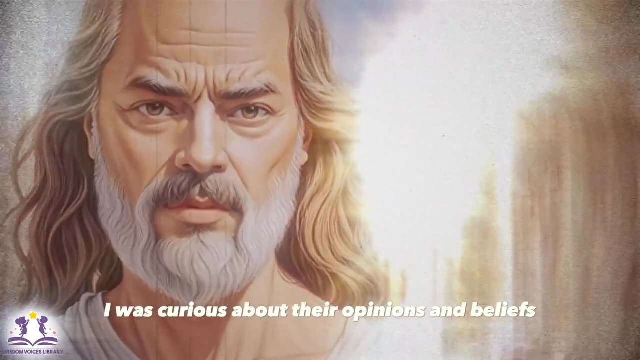 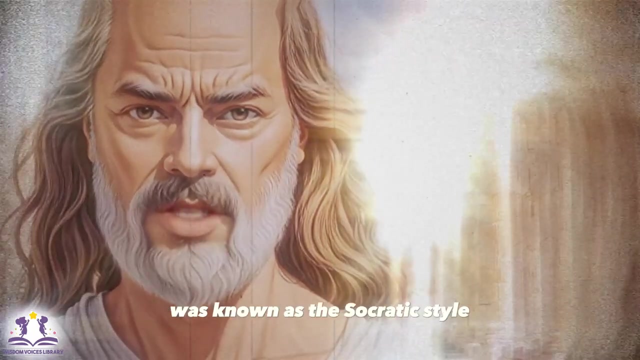 was an effective method of learning. I spoke with folks from various walks of life, wealthy and impoverished, young and old. I was curious about their opinions and beliefs. As a result, I learned that everyone had something worthwhile to offer. My most well-known teaching style was known as 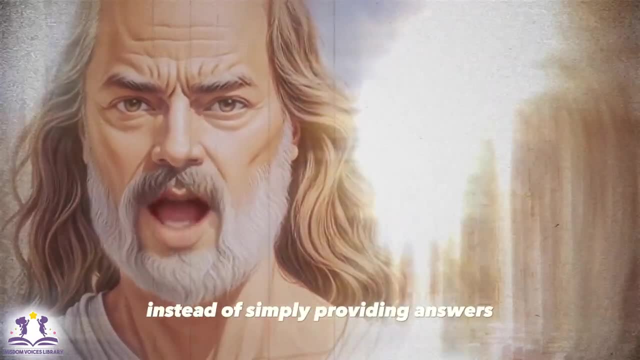 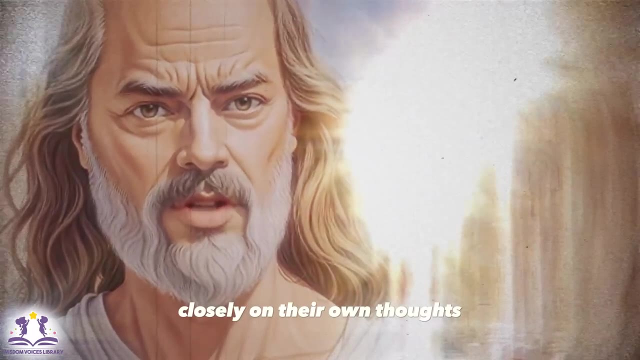 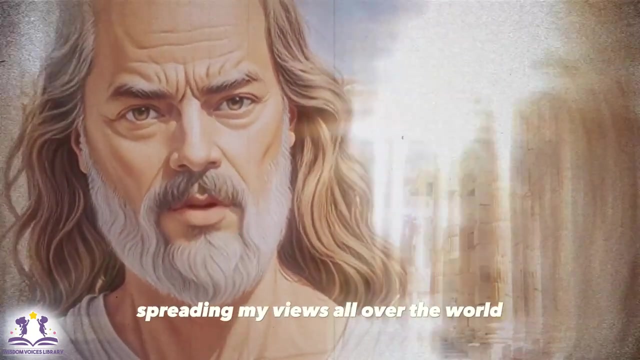 the Socratic style. Instead of simply providing answers, I would pose thought-provoking questions to my students. This caused them to reflect closely on their own thoughts. Plato, a young man, became my student. one day, He would go on to become a renowned philosopher, spreading my views all over the world. 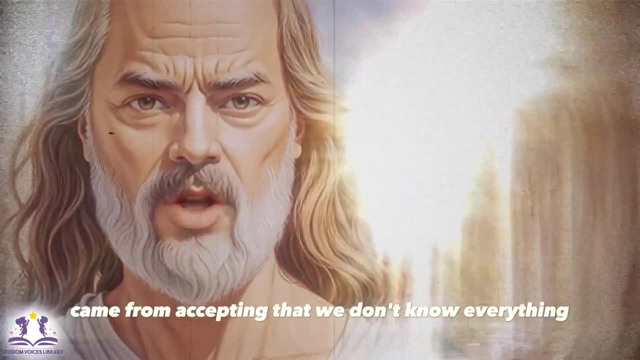 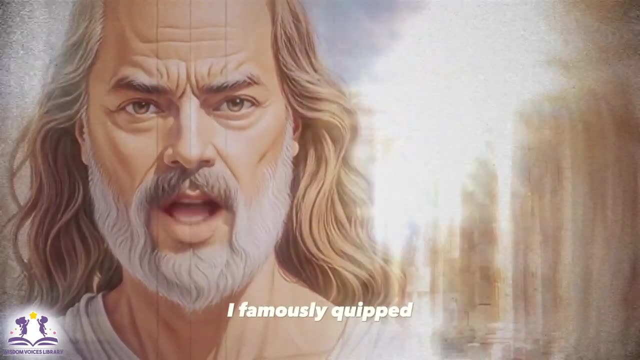 True knowledge, I believed, came from accepting that we don't know everything. Admitting our ignorance allows us to learn. I know that I am intelligent because I know that I know nothing. I famously quipped. Because of my humility, I was able to continue exploring. 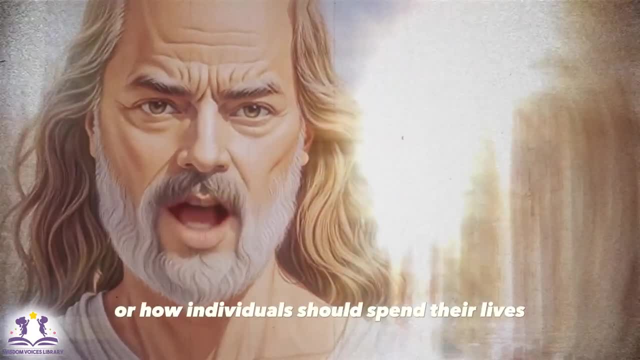 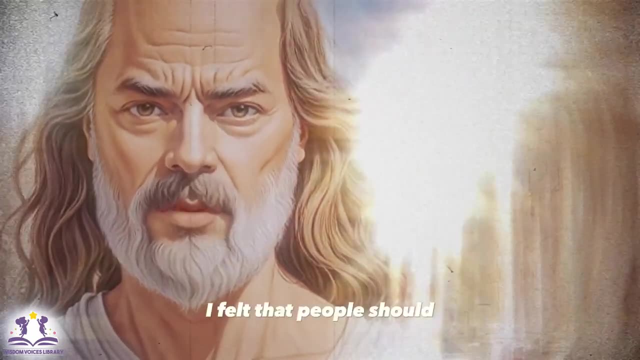 learning and growing. It was also interesting. I was able to learn how to be a good person. I was able to learn how to be a good person. I gave much attention to what it meant to be a good person. I felt that people should constantly. 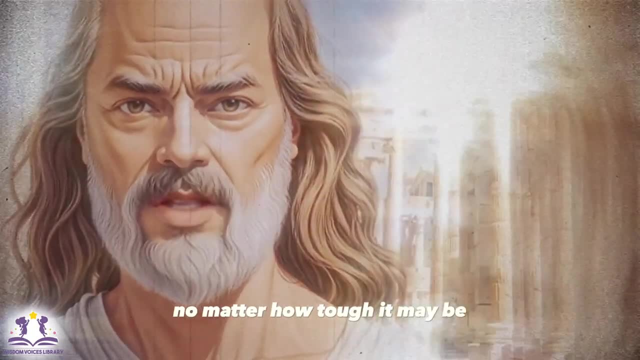 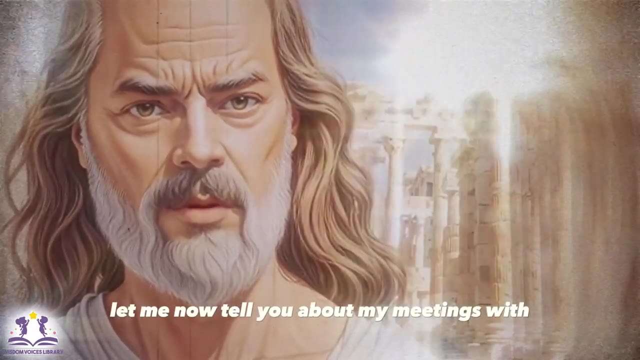 endeavor to do what is right and just, no matter how tough it may be. I urged my friends and students to be truthful, kind and fair in all they did. Let me now tell you about my meetings with the Oracle of Delphi. No one according to this. 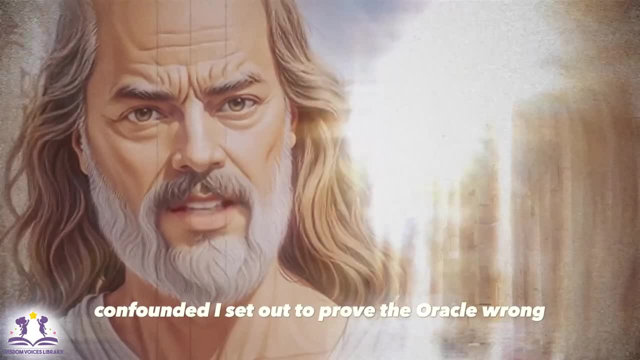 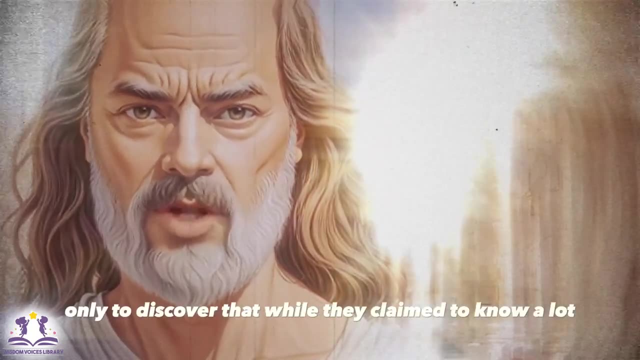 knowledgeable oracle was wiser than me. Confounded, I set out to prove the oracle wrong. chatted with many knowledgeable people. I was able to learn from them. I was able to learn from them. I was able to learn from these mysterious people- politicians, poets and craftspeople- only to discover that 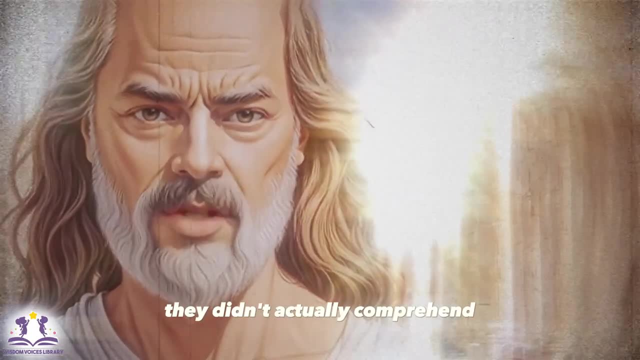 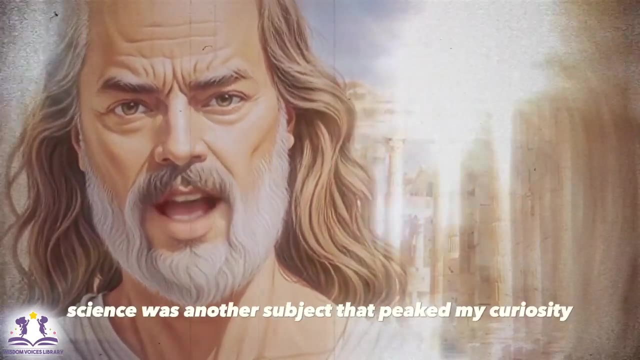 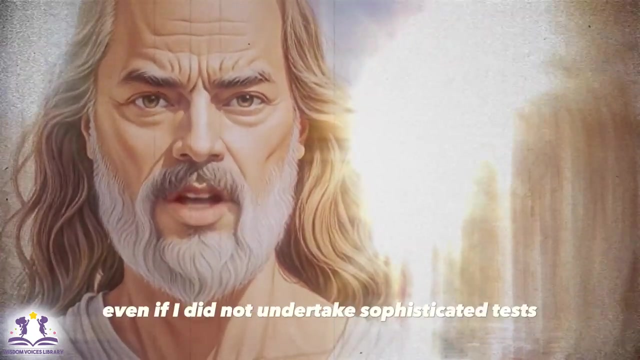 while they claimed to know a lot, they didn't actually comprehend the breadth of their knowledge. This adventure strengthened my conviction in the need of inquiry and humility. Science was another subject that piqued my curiosity. I believed in exploring explanations for the natural world even. 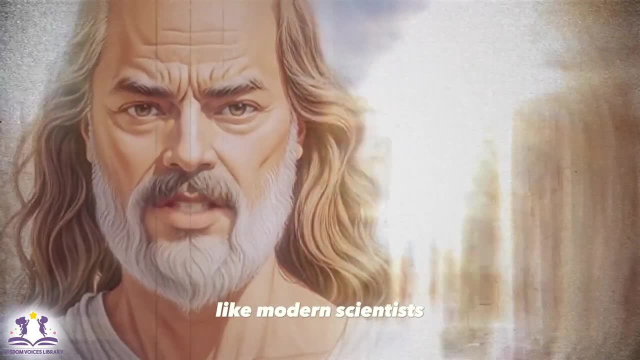 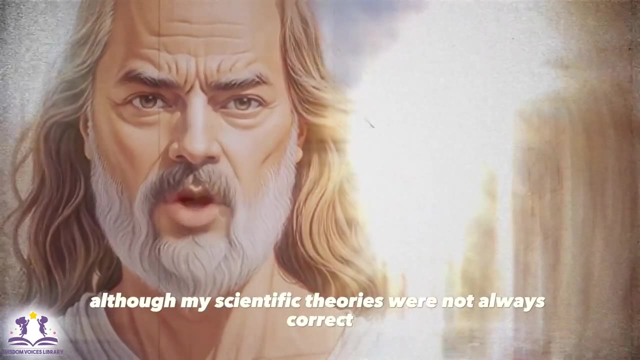 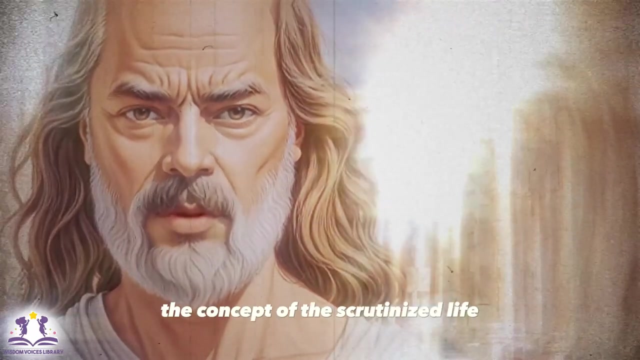 if I did not undertake sophisticated tests. like modern scientists, I considered the stars, the seasons and the natural wonders. Although my scientific theories were not always correct, my curiosity and eagerness to learn prepared the way for future scientific breakthroughs. The concept of the scrutinized life was one of my favorite ideas.